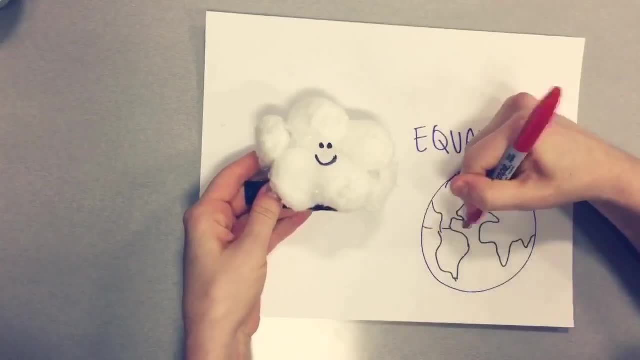 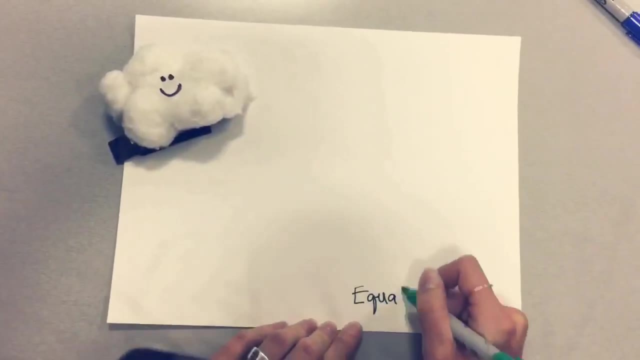 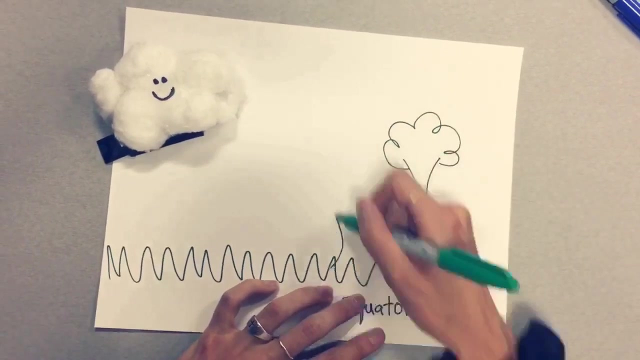 Hi guys, I'm Hadley. I'm a cloud that is created at the equator. I'm responsible for the trade winds in the tropics and I control the low latitude weather patterns. How Well I'll show you First. I'm a cloud that forms at the equator, which is at zero degrees latitude and is home to most of the tropical rainforests. 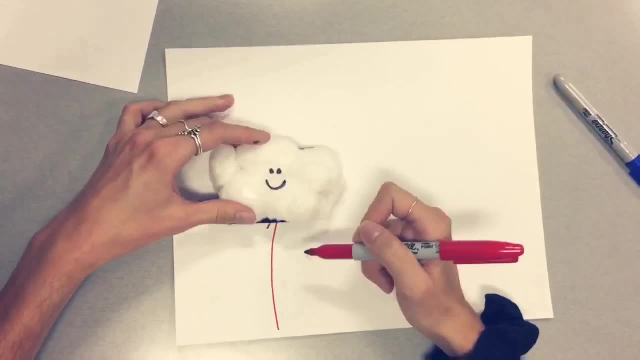 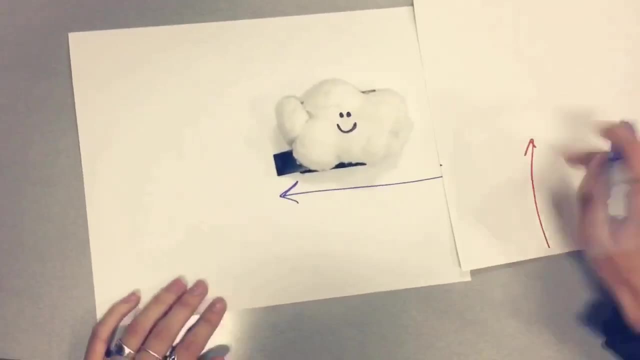 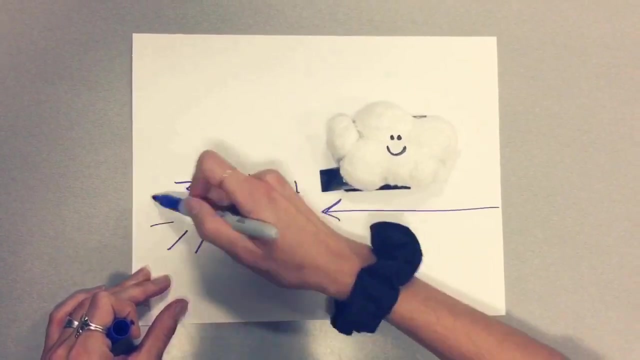 I then rise because warm, moist air rises. It is perceived to be auana fluid in air moving from north to south at the equator. when I'm shortly behind the equator, Air moves towards the poles around 30 degrees north and south of the equator. 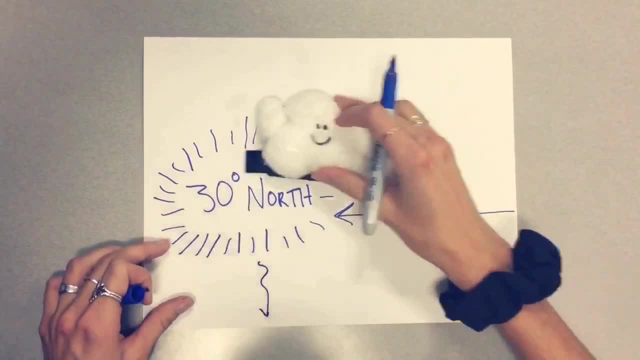 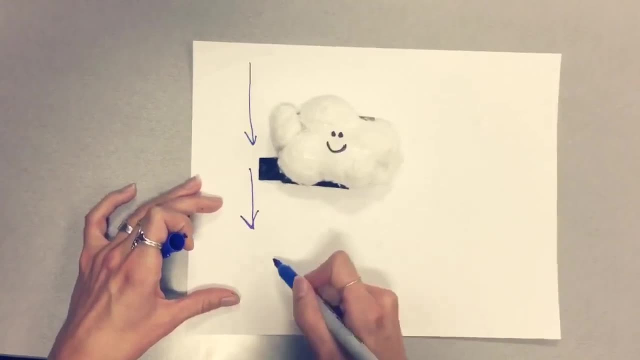 I'm reporters and now I'm just some of the brackets in a Chinese called geological�동. At this point, the air becomes cool and dry at the higher latitude and I begin to sink. Right now, water grabbed a heatex, after which the ground started to sink. 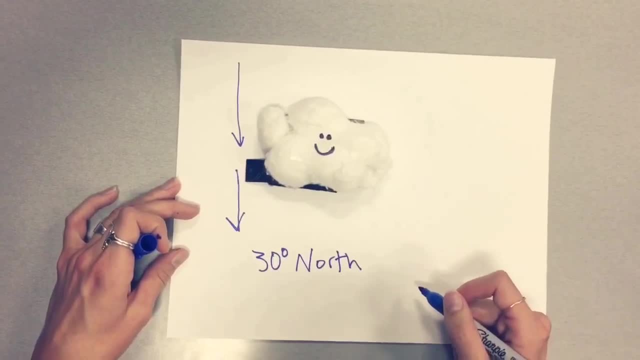 Water moves dry at higher latitude and I begin to sink. I sink because as the air cools, it becomes more dense at my height and height, and so I sink back to the earth around 30 degrees latitude. Because of this, I flow back towards the equator, close to the earth's surface. 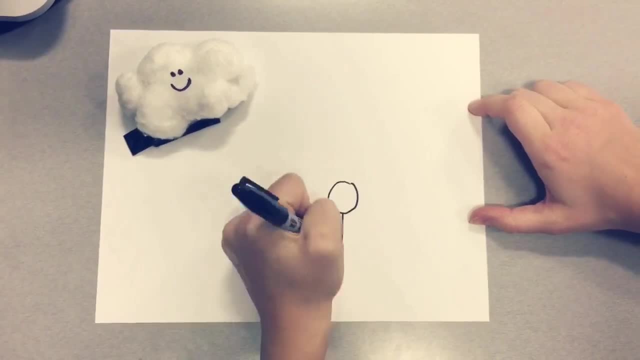 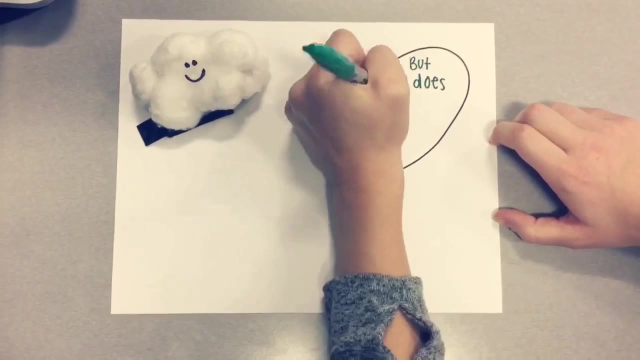 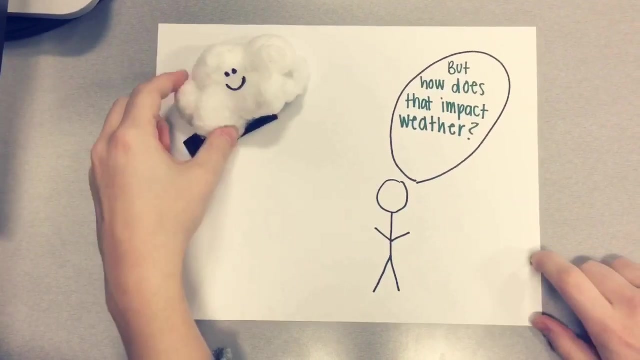 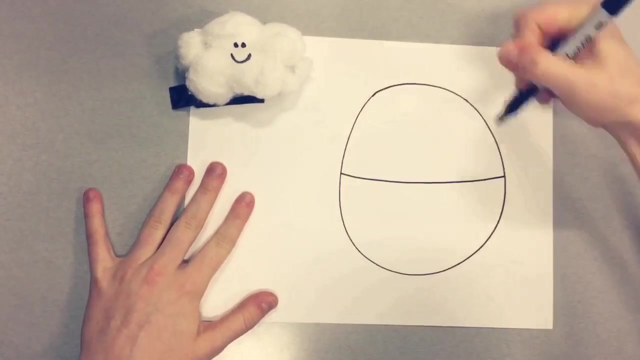 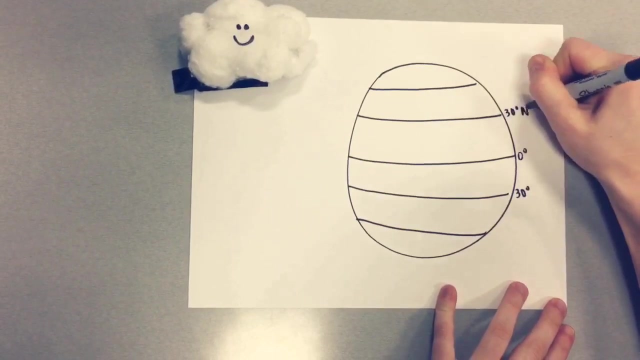 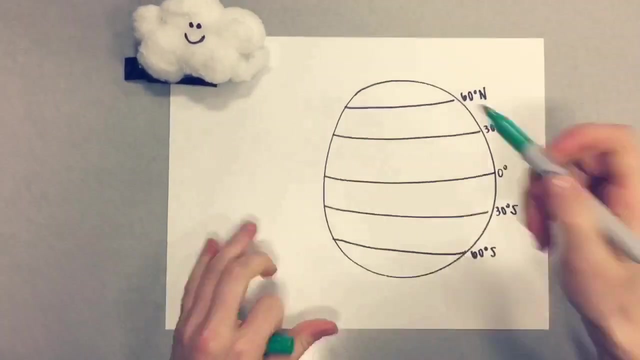 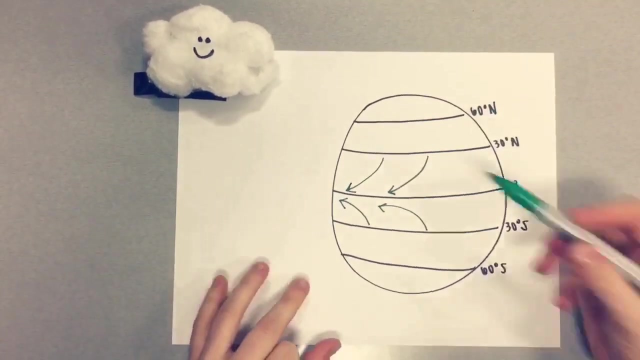 When the air gets warm again, I can start over. But how does that impact weather? Awesome question. I move north and south of the equator and I do that through the use of rising and sinking air. These powers are very powerful.